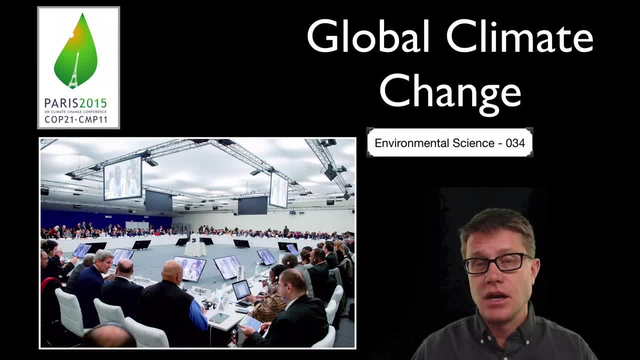 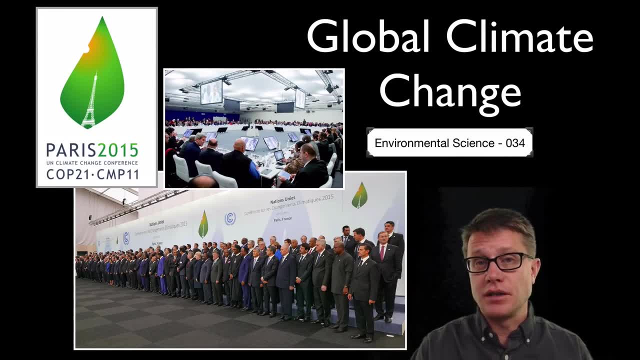 meeting over the last two decades at the UN climate change conference as a way to figure out how we can reduce these greenhouse gases. The first protocol was the Kyoto Protocol And then, more recently, in 2015, is the Paris Agreement. You can see right here, President. 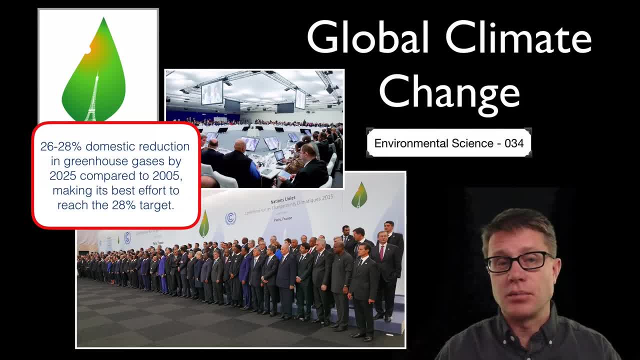 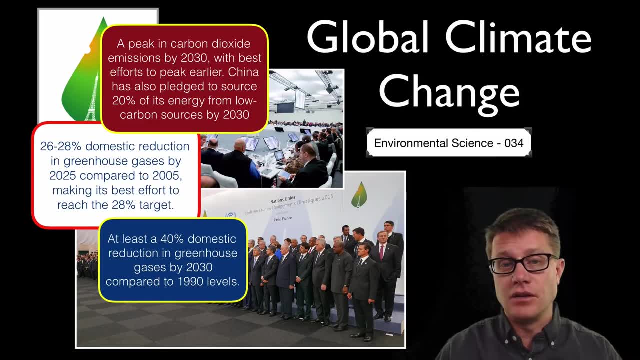 Obama in the middle. The US pledged for a 26 to 28 percent reduction in greenhouse gases. China is going to peak their carbon dioxide by 2030.. 40 percent reduction in the EU, 37 percent reduction in Brazil. But these 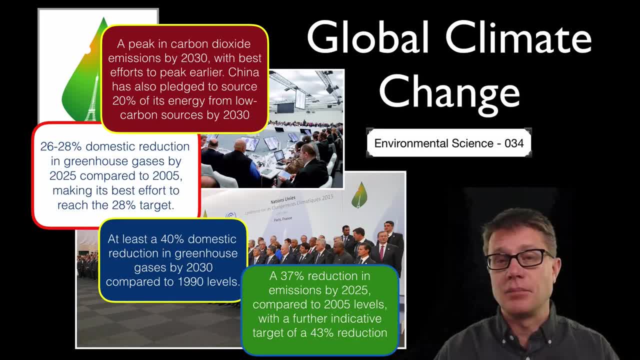 are all simply pledges that they have agreed to. They are not legally binding. The only thing that is legally binding is we are going to start monitoring the greenhouse gases, And so we will see how that plays out over the next 5 to 10 years, And so the climate. 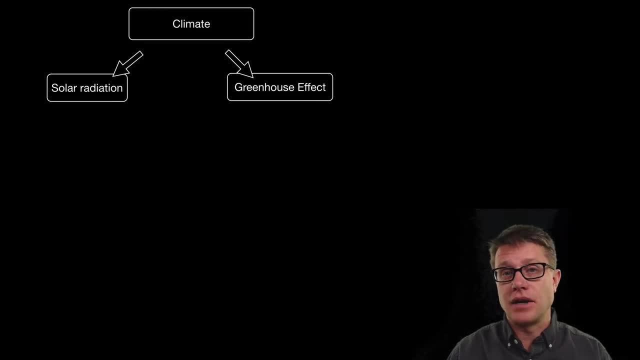 is affected by the solar radiation and the greenhouse effect And as those change, we get global climate change, Which can impact the environment and therefore can impact the humans. The problem we have right now is it is getting too hot too fast. We cannot really affect solar radiation, so we look to the greenhouse gases as a culprit. The five: 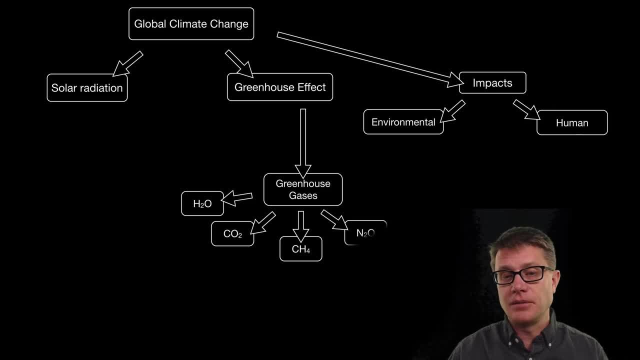 different ones that we will talk about are water, carbon dioxide, methane, nitrous oxide and then CFCs. What they do in the atmosphere is they essentially trap infrared radiation. Some of these sources are natural, So volcanoes, for example, are going to put carbon dioxide. 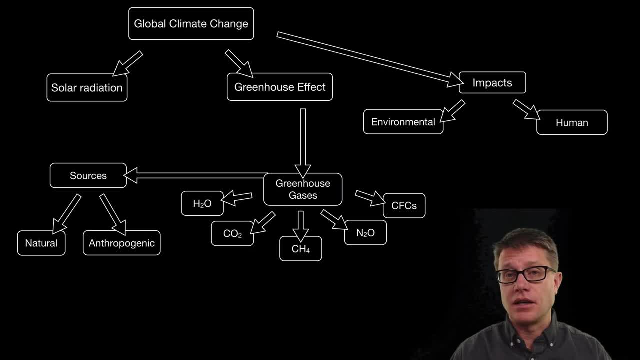 or water vapor into the atmosphere. But a lot of these are anthropogenic, In other words, we are producing these and they are warming up the planet, And so treaties are being signed to reduce the amount of greenhouse gases in the atmosphere, to kind of mediate. 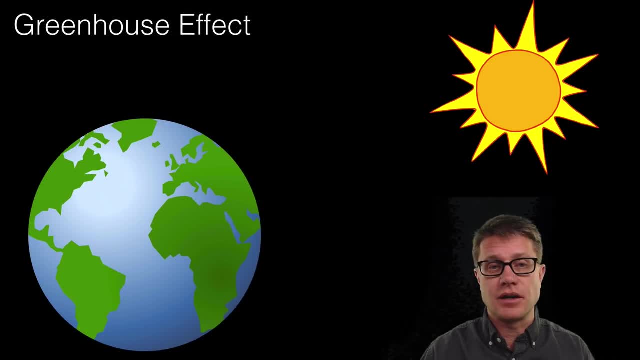 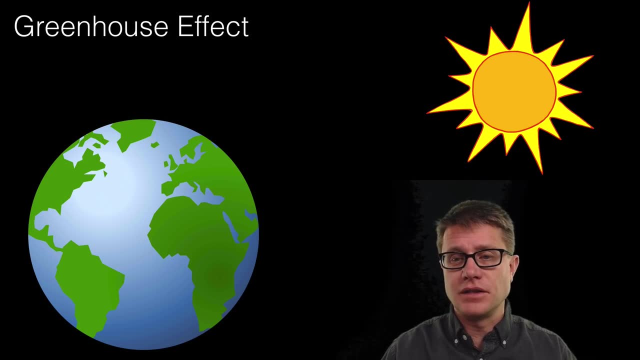 some of these human impacts. Kyoto Protocol and Paris Agreement are two that we will talk about. So how does the greenhouse effect work? Well, let's say that the earth did not have an atmosphere, And clearly this model is all off. But if it did not, then light would come. 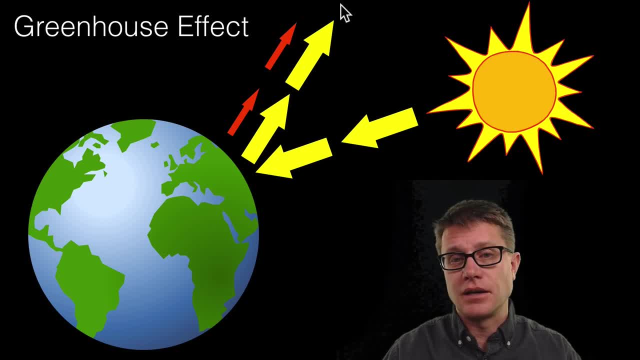 from the sun, It would hit the planet. A lot of that is reflected back into space, But some of it is converted into infrared radiation. It also would go into space, And so the earth would essentially be a ball of ice. There would not be enough heat to heat the planet. 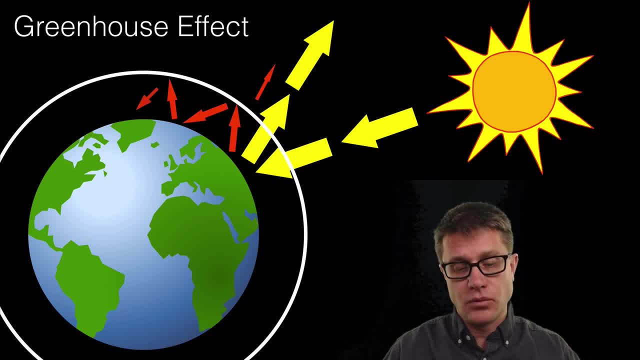 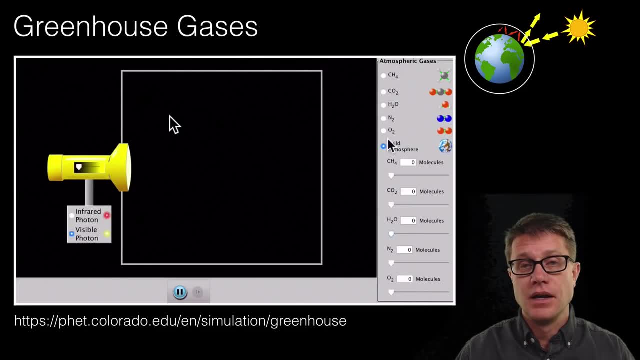 And so what happens with an atmosphere is that we trap that. So once it hits the planet, that heat is left behind, And so it warms it up. It works just like a greenhouse does on a warm day. So if we look more specifically at what is going on with the greenhouse gases, 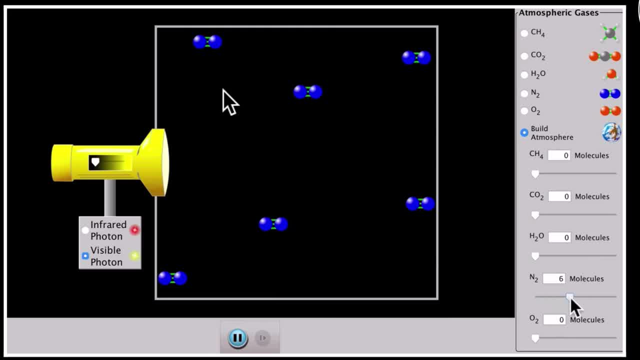 this is a PHET simulation, And so what I am going to do is I am going to create an essential atmosphere, So I am going to put a little bit of methane in here, And then I am going to put a little bit of nitrogen in the atmosphere. We are going to put some oxygen in the atmosphere. 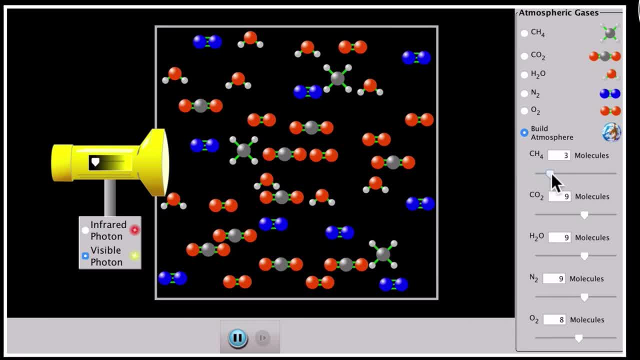 We are going to put in a little bit of water vapor in the atmosphere. Now we have got some carbon dioxide And finally we have some methane. So this is our pretend simulated atmosphere, And as light moves through it, you can see that it is not interacting with any of those. 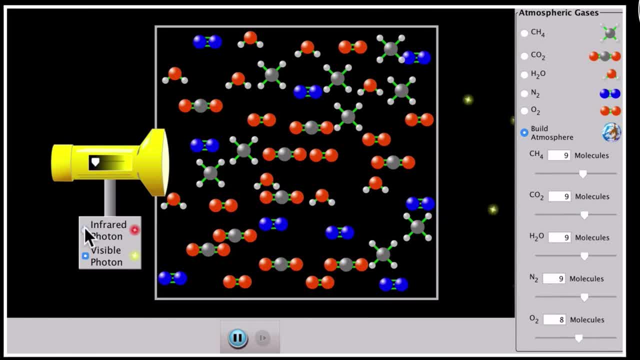 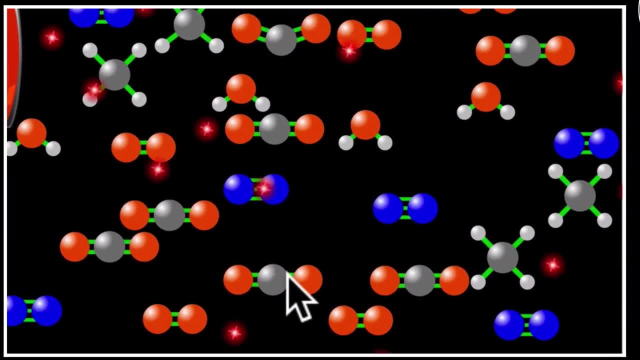 gases. That is how the light gets through the atmosphere to our planet. Once it hits the planet, it converts to infrared radiation. Watch what happens as that starts to leave the planet. You can see that some of these are refracting some of that infrared radiation Instead of 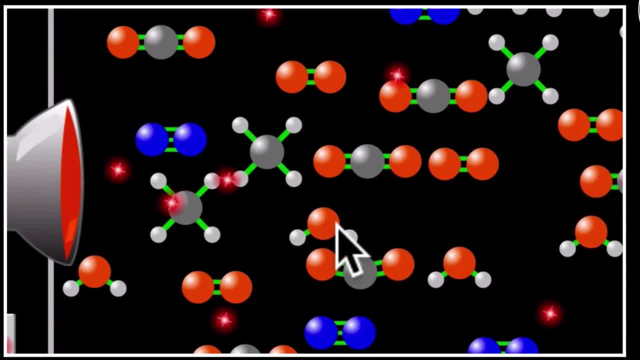 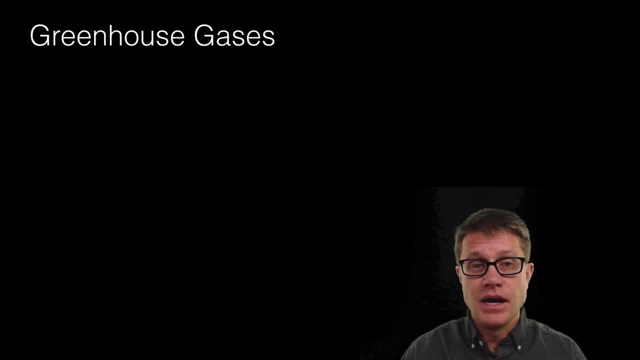 moving back into space, it actually returns. What are those greenhouse gases? We can see methane, We can see water, We can see carbon dioxide, But the oxygen and the nitrogen are not impacted at all, And so greenhouse gases are water vapor, carbon dioxide, methane. 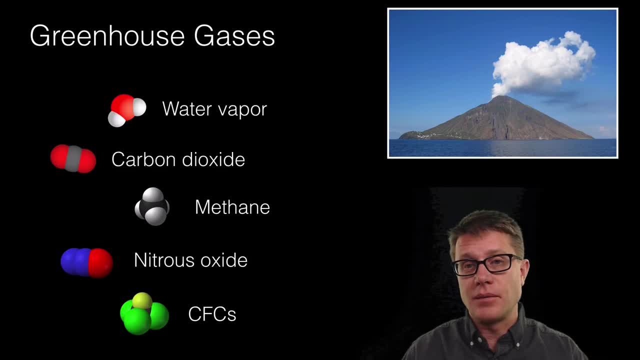 nitrous oxide and CFCs. These are molecules in the atmosphere that trap that infrared radiation. A lot of those are made through natural processes, And so carbon dioxide is produced. in a volcanic eruption like this, Also, a lot of sediment moves into the atmosphere. 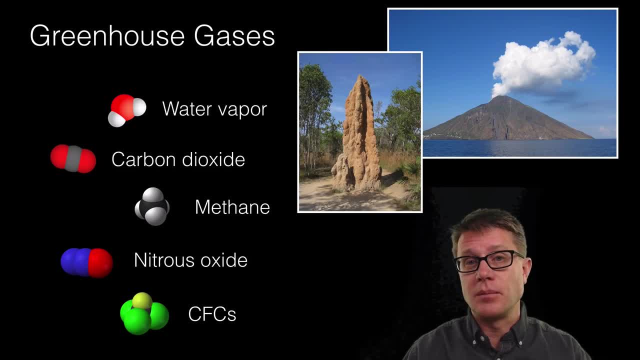 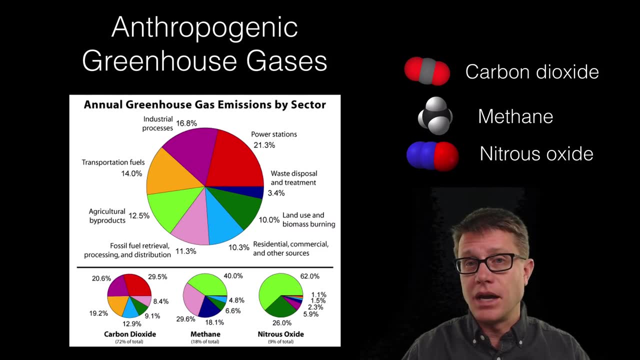 which will actually cool the planet from a volcano, Or this giant termite mound is going to produce methane gas that goes into the atmosphere. The problem is that a lot of these are anthropogenic. In other words, we are making them, Humans are making them And we are making. 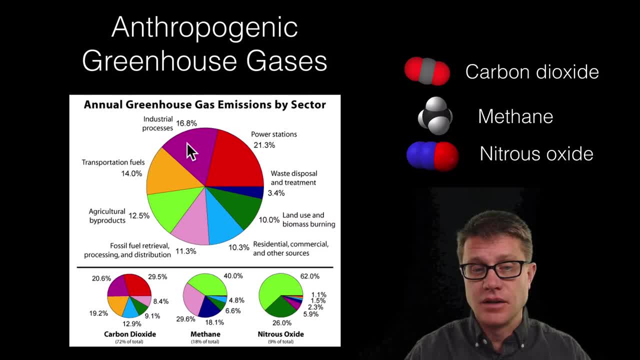 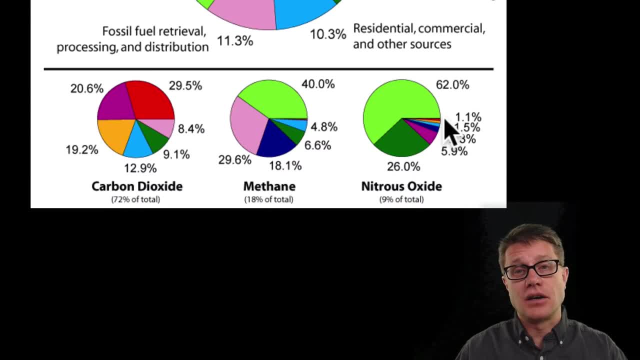 them through agriculture, through power, through industrialization. If we look at the three major culprits- carbon dioxide, methane and nitrous oxide- they are produced by different activities on our planet, But all of them are produced by different activities on our. 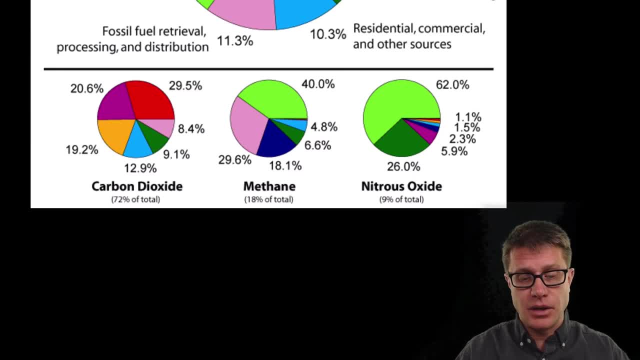 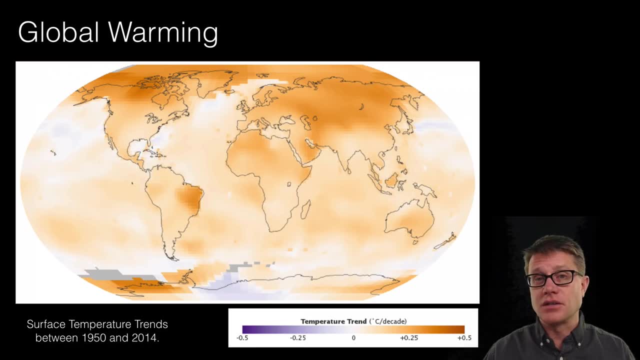 planet, But all of them are produced by different activities on our planet, But all of them are heating our planet. You can see that agriculture impacts a lot of, especially methane and nitrous oxide, And what it is doing is it is warming up our planet. You can see on all parts of 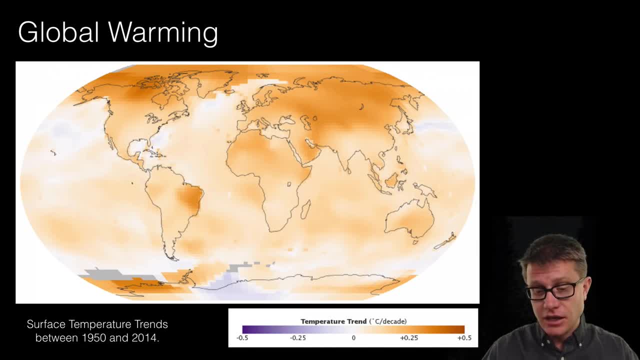 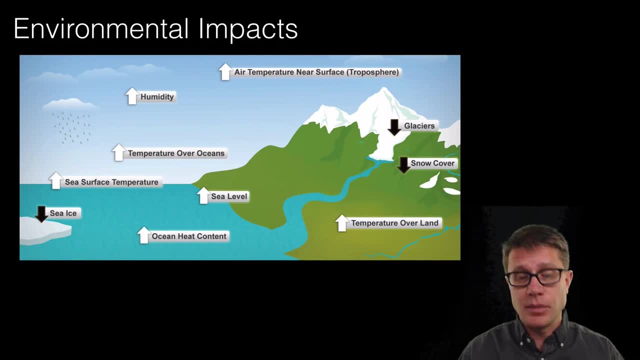 our planet. we are seeing increases in temperature, And some are predicting increases up to 3 or 4 degrees Celsius change over time, And so we have to start to mediate that, Because what happens as we increase the temperature is we are going to get a melting of glaciers. 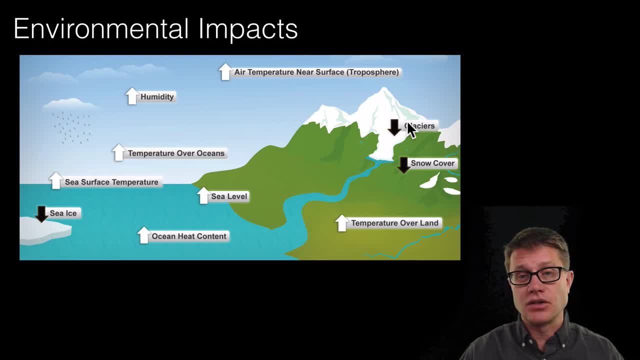 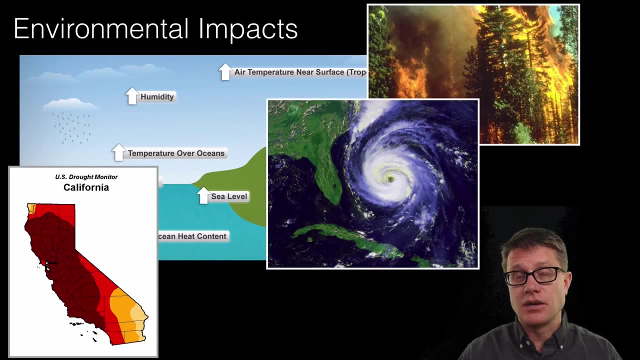 Snow cover goes away, Polar ice caps go away, Sea levels start to rise And, as a result of these environmental impacts, we are going to have human impacts. So we are going to have droughts. Forest fires may increase. The size of the storms are going to get greater. 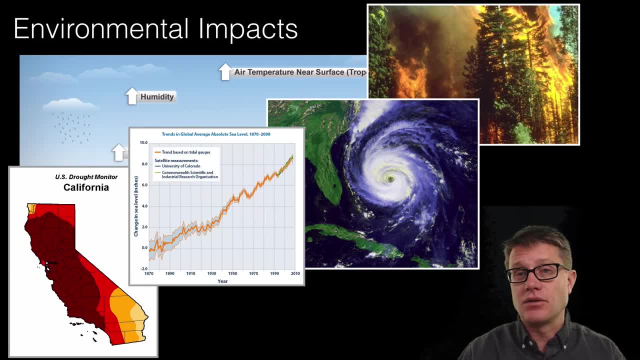 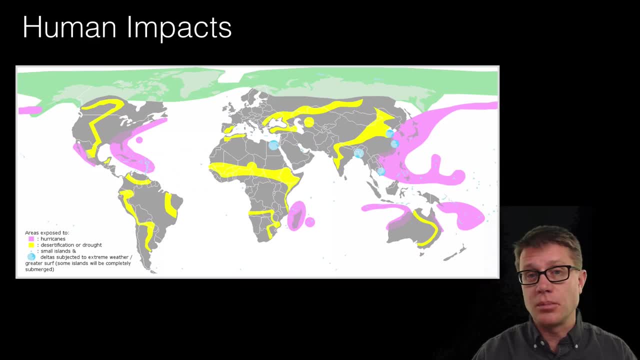 because we are going to have a higher amount of radiation And then we are going to have increases in the sea levels, And so if you live near that coast, it is going to impact you. If we look at human impacts, these are all the planets, humans, that are going to. 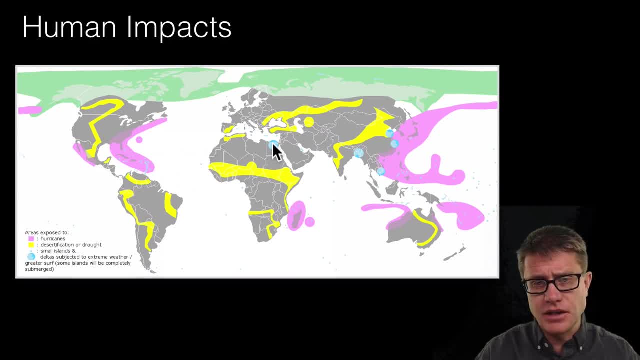 be impacted. If we look at, first of all, the blue, it is hard to see, But all the islands, obviously, as the sea levels start to rise, are going to be impacted, Especially if you live around these deltas. All these purple areas are going to be hurricanes, All these. 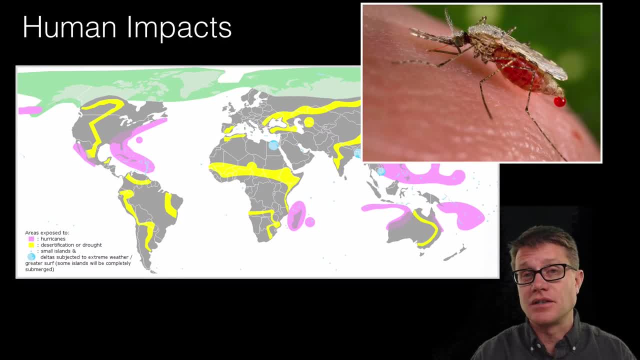 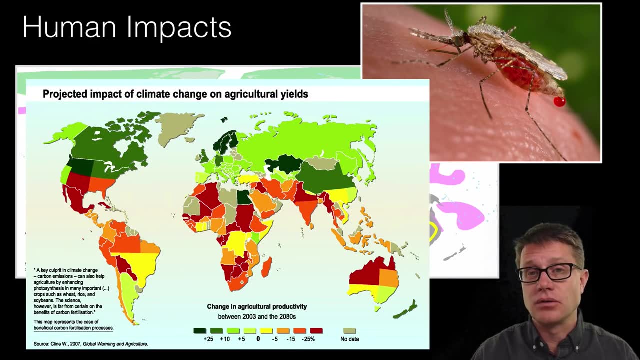 yellow areas are going to be droughts. We are also going to see changes in disease. Malaria is going to start to move to areas where it was never found before. Those droughts are going to lead to decreases in agricultural yields and that is going to impact humans. 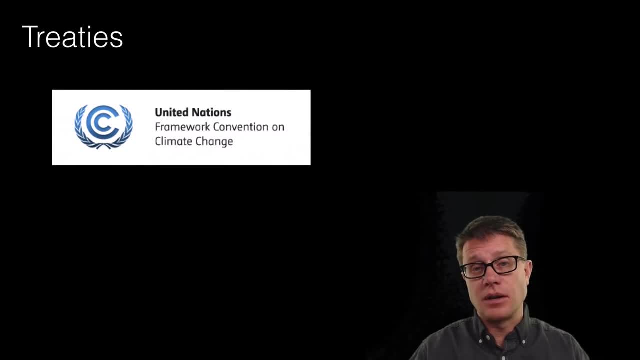 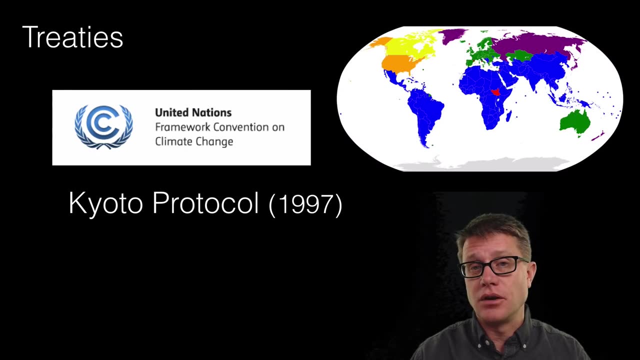 as well. And so what do we do? Countries are coming together. This is a global problem. No one owns the atmosphere. We all own it together, So we have to work together, And so the first was the Kyoto Protocol. It was thewegen of a fearsomeilia. We realized that. 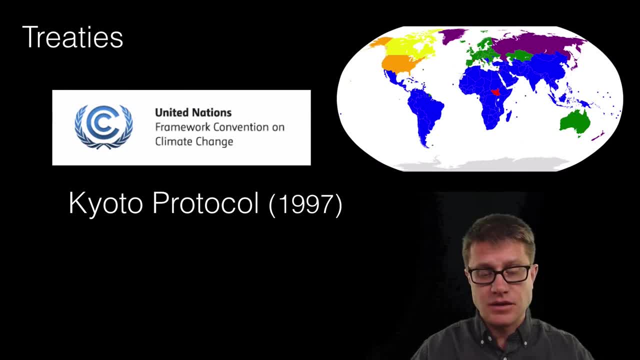 looking around we found around each of those places could be the biggest problems with all. It was a reduction in greenhouse gases. You can see that only the green countries were legally binding to reducing the amount of greenhouse gases. A lot of them were not legally bound. The US did not ratify it. Canada pulled out after a year, 2015 again. we have 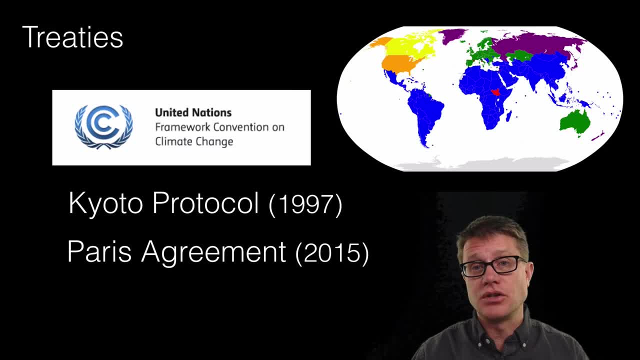 the Paris Agreement, where all these countries are making pledges on reducing the amount of greenhouse gases And the goal is to keep that change on our planet under 2 degrees Celsius as we go into the next century. But it is going to require us kind of to work. 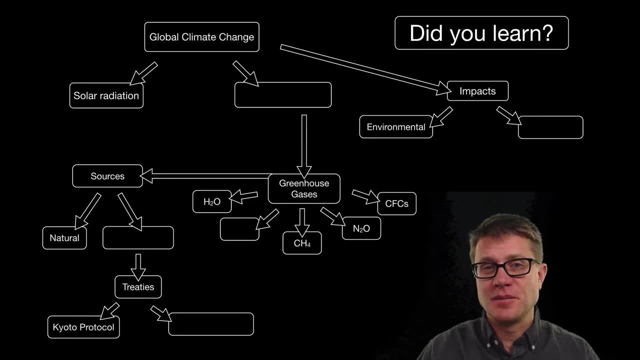 together. So did you learn the following? Could you pause the video and fill in all the blanks? Let me do that for you. Global climate change is affected by solar radiation and the greenhouse effect. It is going to cause human impacts- The greenhouse gases. 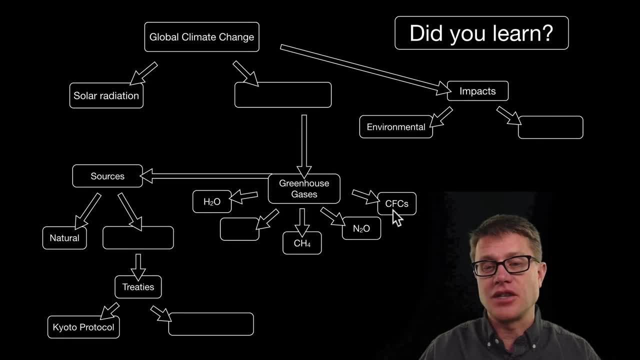 are water vapor- Carbon dioxide is the big one- Methane, nitrous oxide, CFCs- Remember. the source of these greenhouse gases is natural and anthropogenic, And so to reduce that we are signing treaties like the Kyoto Protocol and the Paris Agreement. So that is going. 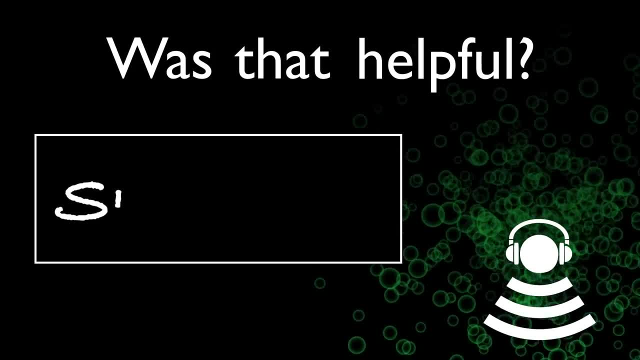 to cost global climate change And I hope that was helpful.